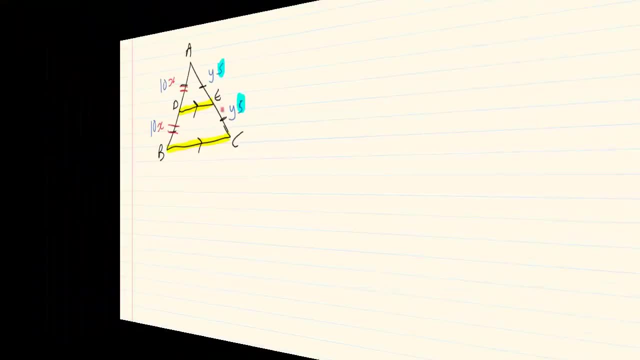 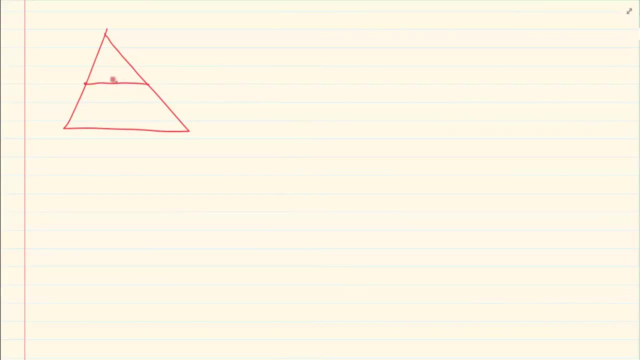 you simplify it, it's 1 is to 1 or 1 is to 1.. Now let us go to your grade 12 theorem. The first theorem you learned said that if I had one side parallel to the other, then this side- if I had x and 3x- would be in proportion to the other side. That is what 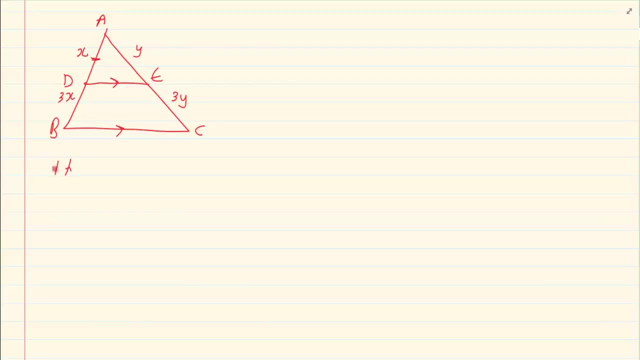 the first theorem you learned said. It basically said that if I had parallel lines, then I had a proportion. So if I had a parallel line, then the sides on the triangle would be in proportion. Now, what is the difference between this theorem? This theorem says that 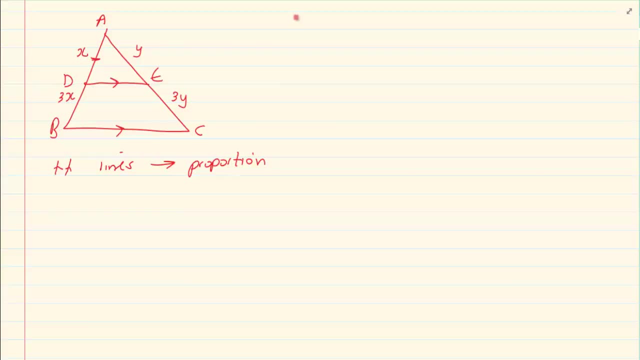 if a line segment joins the midpoint of two sides. Now pay attention to the wording. If a line segment joins the midpoint- Midpoint means middle, So it joins the midpoint of two sides of a triangle. So what is it saying? It's saying that I have a triangle. 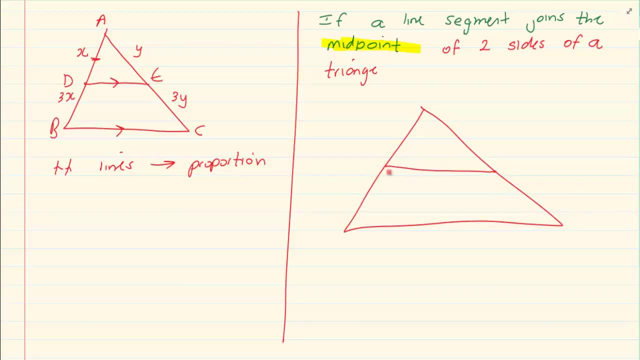 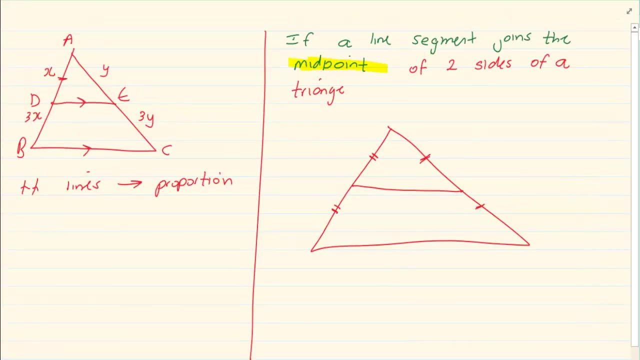 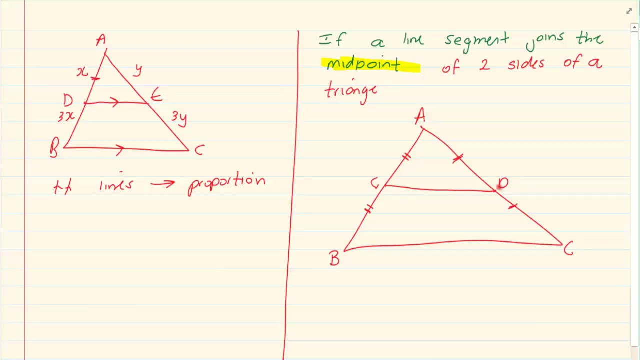 And I have a line segment. But as soon as I put this line segment, it is cutting it in half. Remember, I'm not saying that the lengths are equal. I'm not saying that AE is equal to AD. Neither am I saying that BE is equal to DC. I'm saying that if the line 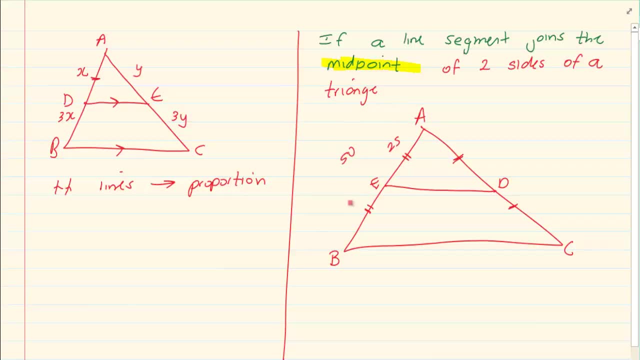 AB was 50., Then it would have cut it into 25 and 25.. Exactly in the middle, If the side was 60, then it would have cut it into 30 and 30. So what I'm saying is it is cutting it in. 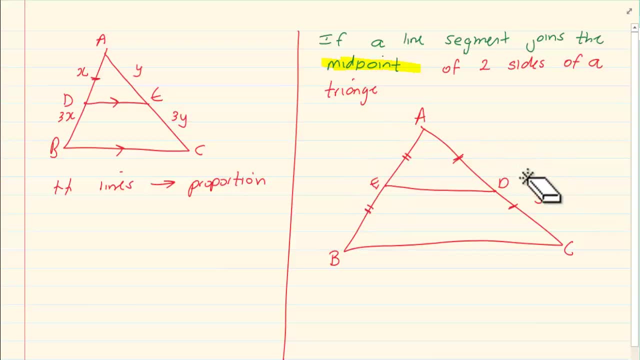 the midpoint. It is not telling me that the lengths are equal. So watch your language. Right N is parallel Right To the third side. So now look, they're giving us one more thing. It's parallel, So it is. 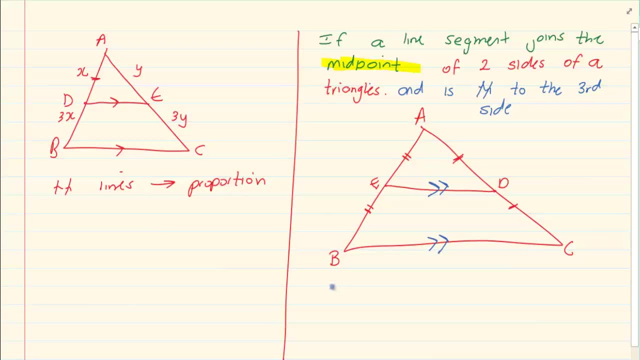 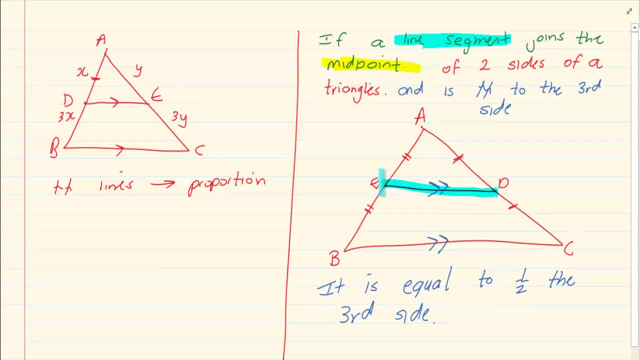 In the beginning. So the line segment in this case is ED. So if a line, let's say ED, joins the midpoint, so it joins the middle of two sides of the triangle and it is parallel to the third side of the triangle, Then it is equal to half of the third side. meaning if 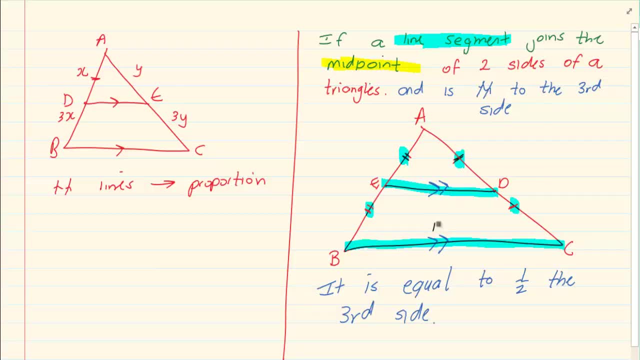 this is 50,, then this would be 25.. If this is a hundred, then this would be 50.. What would you notice? It is always half of the third side, Meaning if this is 2x, half of that would be x. 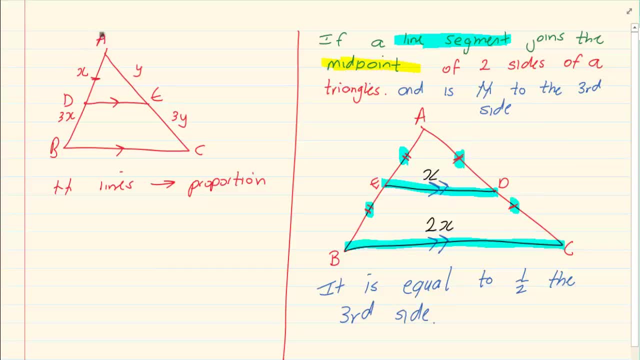 And that is the difference between the theorem you learnt first and the second theorem. Now, what is the name of the second theorem? This is a very famous name. It is called midpoint theorem. Very often we would see that the learners would say midpoint chord. 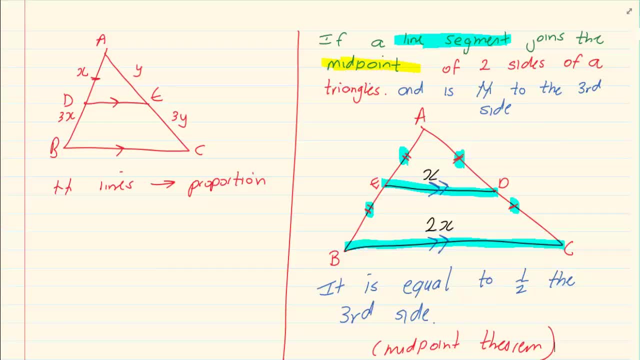 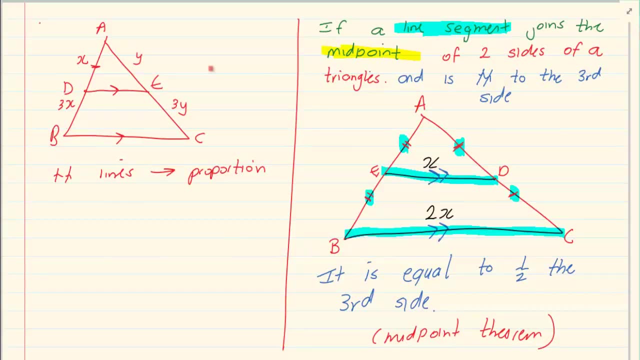 But midpoint chord is not a theorem in grade 12.. There is a difference between midpoint chord and midpoint theorem. If you state midpoint chord, you will be marked wrong. The theorem is midpoint theorem. That is the reasoning, And when we did 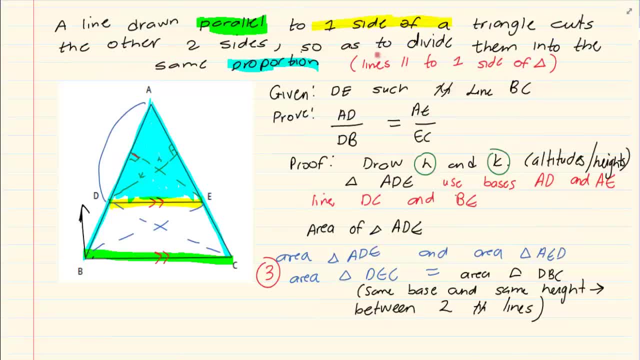 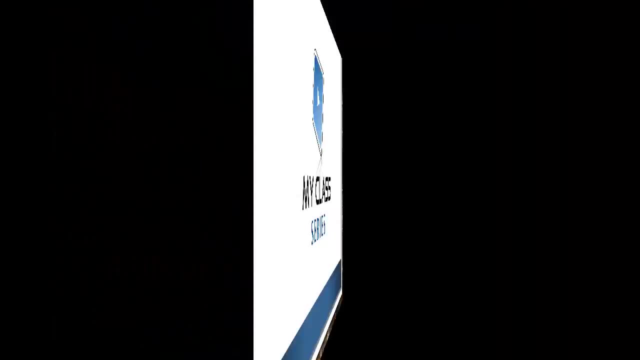 the first theorem, then the reasoning we used was line parallel to one side of the triangle. Thank you for watching. Thank you.